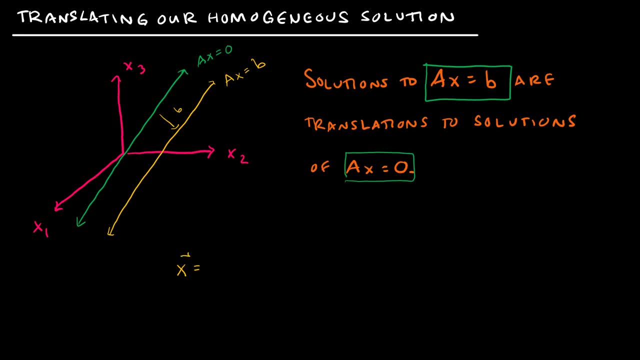 we've been dealing with parametric equations that are in the form either T, V or we also had a situation where it was- excuse me, that's not a plus- where we had T, U, plus. I don't remember S, W, I think are the letters that I used. 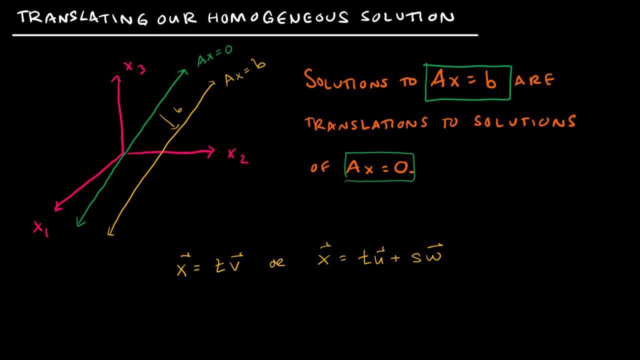 The letters aren't really that important. What is important is we were dealing with some constant times, some vector, or two constants times two vectors, And so that was the parametric form that we're dealing with, And so what's going to change now is we're still going to be able to write it. 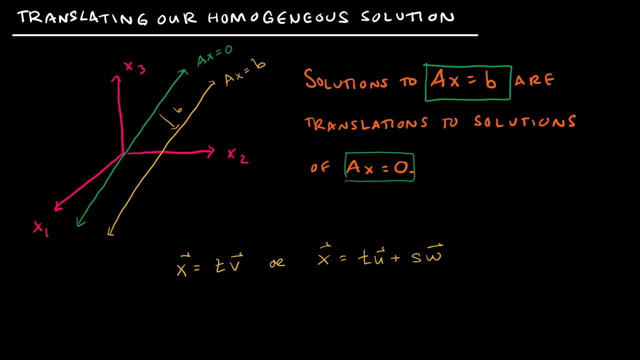 in that parametric form, but what it's going to look like is a little bit different. We're going to end up with something that looks like P plus, say, T, V, And again, this is that same solution as I would have had for a homogeneous solution. 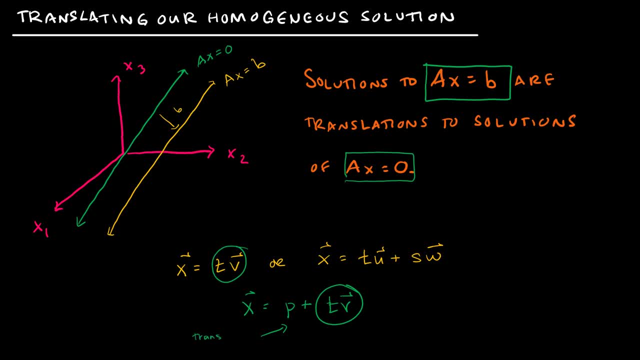 And P is going to be whatever my translation is. So of course it makes much more sense when we actually do this together. And again, I've drawn one with a line. It would be the exact same thing if ax equals zero. the solution set was a plane. 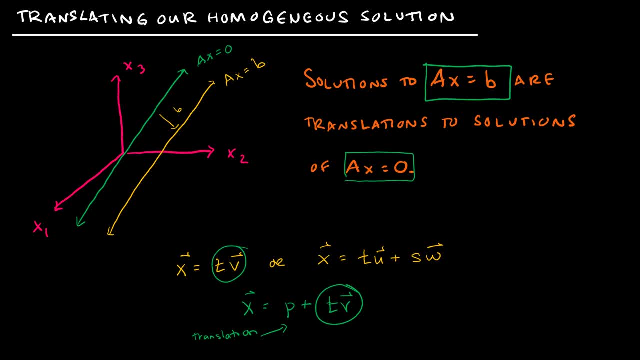 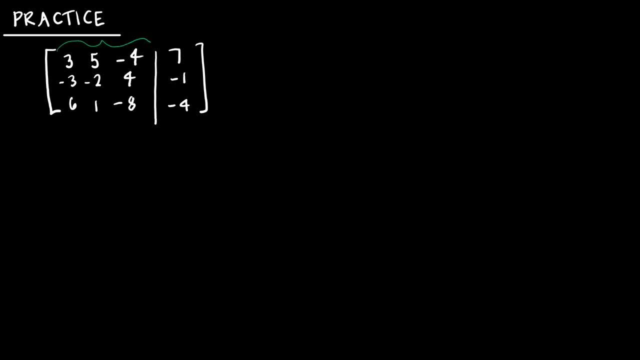 it would still just shift the plane b units. So let's look at this one together And, if you'll notice, the coefficient part of my matrix should look familiar because I reused these numbers from example that we did in our last video. But, if you'll notice, this is not homogeneous. 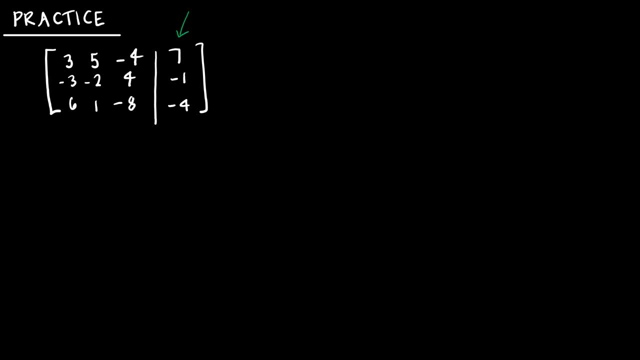 because this row, or sorry, column, is not zeros, So it is not homogeneous. But the good news is we're going to just do the same steps that we would do when we did this for a homogeneous system. So I still want my first row. 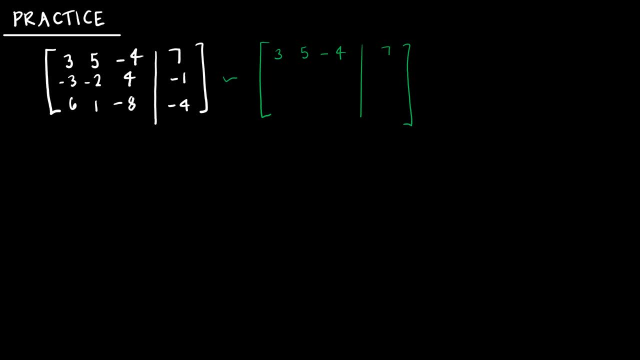 to remain the same. because I want this three to be a pivot, I'm going to add rows one and row two to give me my new row two, which gives me zero three, zero six. I'm going to take negative two times row one. 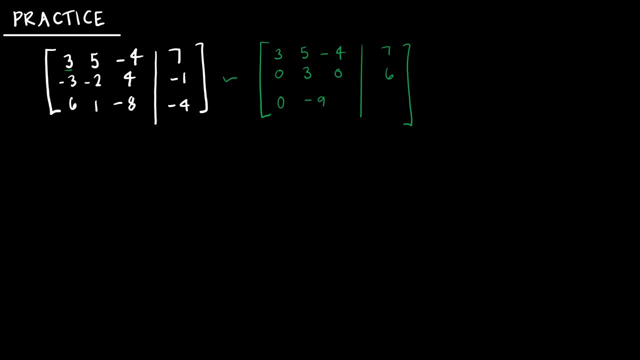 and add it to row two to give me zero, negative nine, zero, negative 18.. From here I want three to be a pivot, so I need to make negative nine and two zero nine. So I'm going to take negative three times row one and add it to row two to give me zero, negative nine, zero, negative 18.. 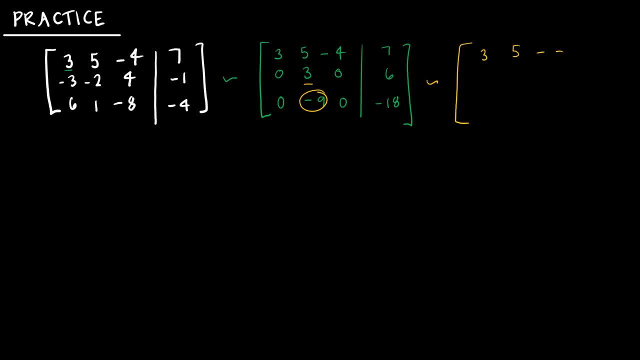 0.. So 3, 5, negative, 4, 7, 0, 3, 0, 6.. And I'm going to take negative- I'm sorry, positive- 3 times row 2 to add to row 3.. So that gives me 0, 0, 0, 0.. So again we can see that X3 is free. 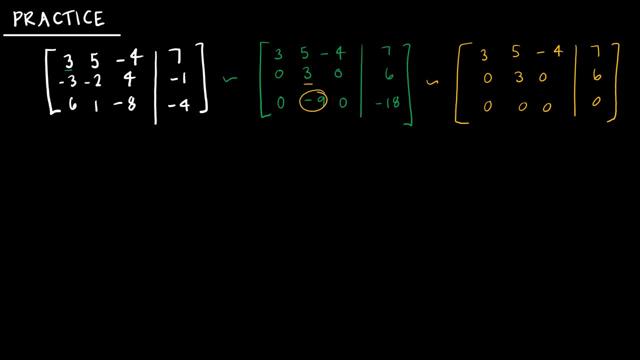 I'm going to continue with my row operations so that I can get this guy to be a 1, and then this guy to be a 1 and this guy to be a 0. Because, of course, that's what we want. So first I'm just 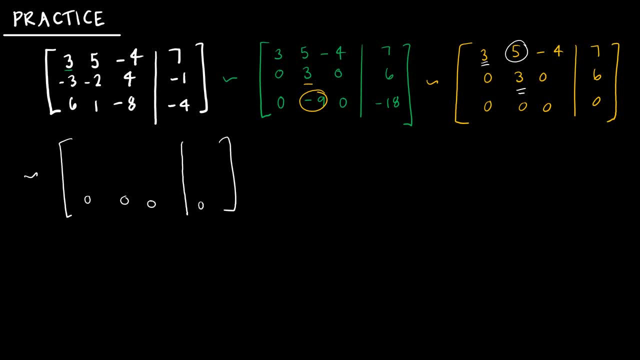 going to rewrite my zeros down here And I'm going to take- I'm just going to do this in two different steps- I'm going to take a third of this And I'm going to keep this guy the same, And then I'm going to take negative 5 times row. 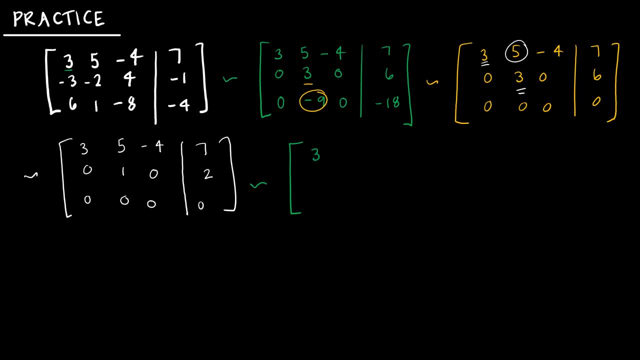 2 plus row 1.. So that's still 3.. Oops, I should go ahead and rewrite these, Otherwise I confuse myself. So negative 5 times 0 plus 3 is 3.. Negative 5 times 1 plus positive 5 is 0.. Negative 5 times. 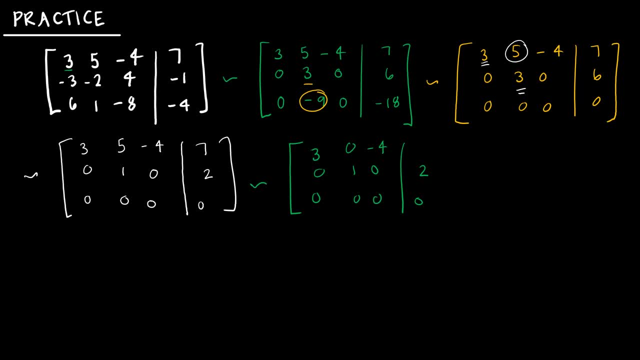 0 is 0 plus negative 4. And negative 5 times 2 is negative. 10 plus 7 is negative 3.. So far I like what I'm seeing, And the last thing I want to do to make this just a little bit prettier is to just take a third of. 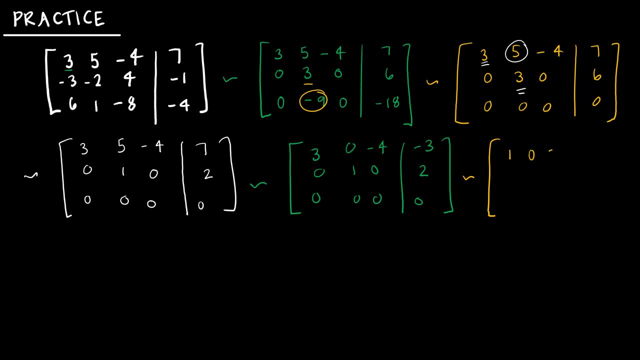 row 1.. So this is 1, 0, negative 4 thirds negative 1.. This guy remains the same, And this guy remains the same. So this is where we are now And we can see. this looks very familiar. The only difference. 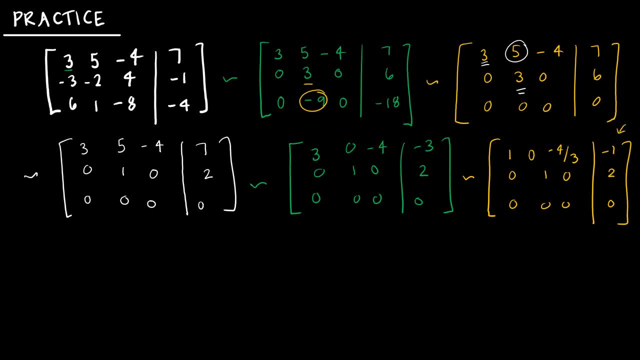 here is the fact that these guys aren't all the same. So I'm going to take a third of this And I'm going to rewrite this, because in this row you're going to have all the zeros, And before they were all zeros. So how is this going to change what I do next? Well, remember before I. 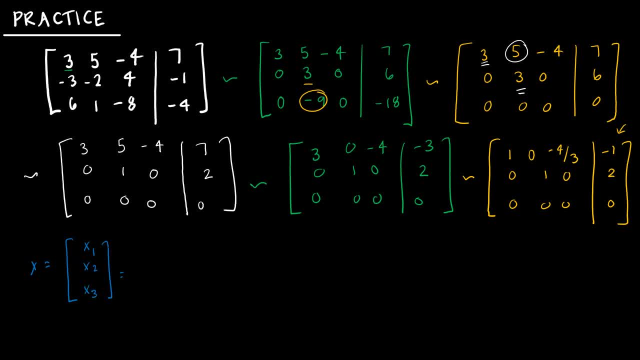 wrote this as x1, x2, x3. And that's really what I'm going to do again. So this guy is x1, minus 4 thirds x…. Let me just go ahead and write that before I get into my matrices, just to make sure we. 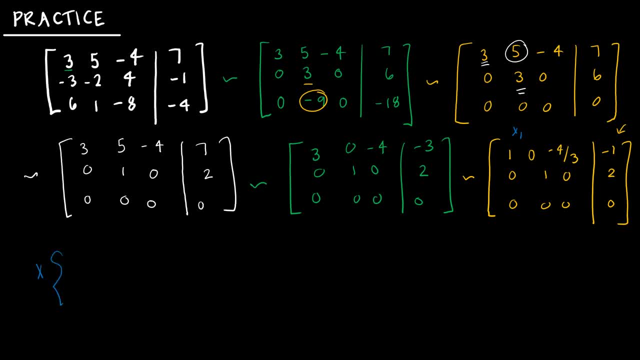 don't have any misunderstandings. So my solution- wow, my solution set- is x1 minus 4 thirds. x3 equals negative 1, I've got. x2 equals 2, I've got x3 is free. And so what I'm going to do now is I'm just going to write that in a different format. 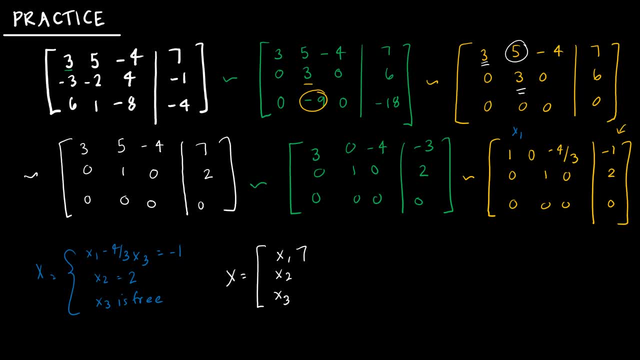 x1, x2, x3.. So x1, if I rearrange this would be negative 1 plus 4 thirds x3.. X2 is 2, x3 is just x3.. So that's where I stand right now is this is my solution. 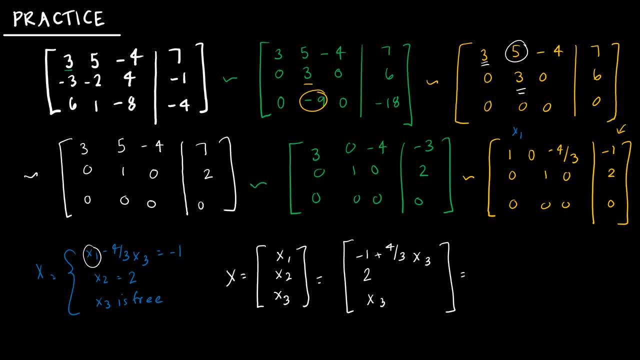 And what I want to do is: I want to write this. I hopefully don't run out of room here. I want to write this in two different vectors. I'm going to have my negative 1 and my positive 2, and notice there's nothing else here. so 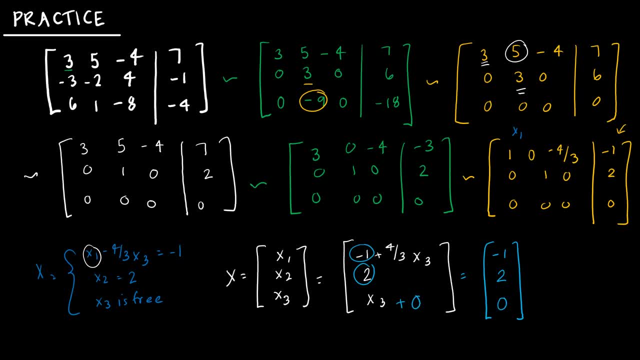 that's essentially 0.. And then my other matrix is going to have an x3, so all of the x3 terms. So I'm going to factor the x3 out And so that's going to give me 4 thirds. nothing here. so that's a 0. 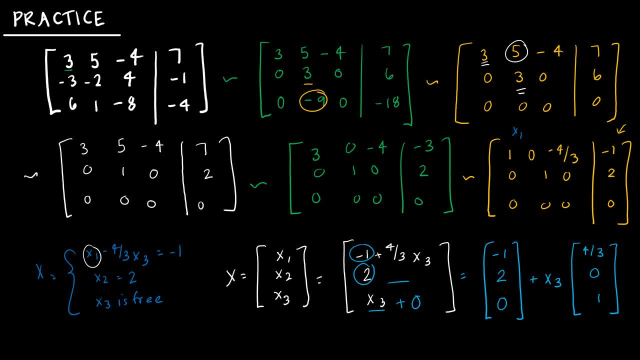 And then a 1.. And so, again, did I write this in the format that I wanted? Well, if you'll recall, in my last slide we talked about that. we wanted x to be p plus tv, And did I accomplish that? 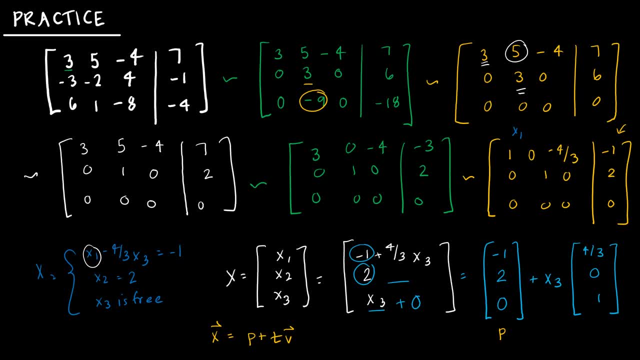 Well, this is p and that's my translation. This is t and this is v, So I did accomplish it. I wrote it in the format that I wanted And again, p is simply the translation of our homogeneous solution of tv. 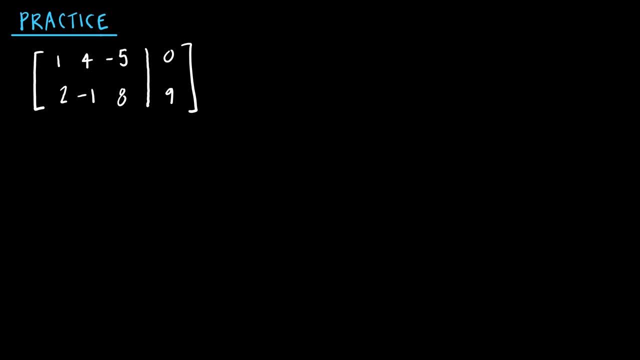 Here's a practice for you to try on your own, so go ahead and give it a shot. When you are done, press play to see how you did. As you can see, this is a non-parametric equation, because I don't have all zeros here. 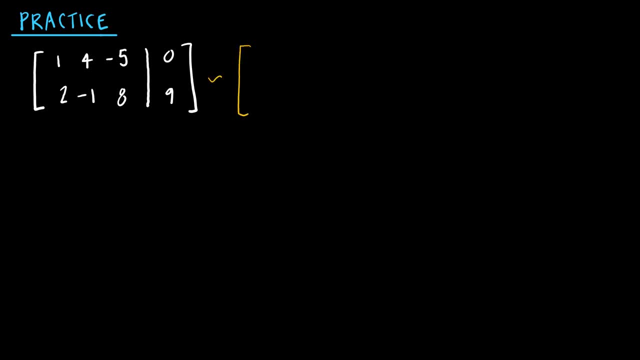 So let's go ahead and do the same thing we did last time with those row operations. Again, I've got a pivot here of 1. And so I want everything below that pivot to be 0.. And so I'm going to take negative 2 times that first row and add it to my second row. 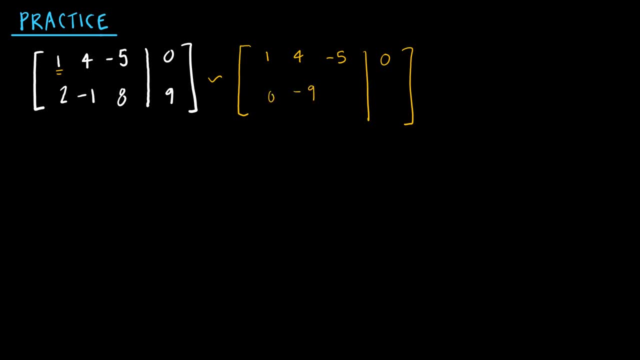 So that's going to give me 0, negative 9,, positive 18, and positive 9.. And now I want this guy to be my pivot, And so, again, I'm looking for reduced row echelon form. So I'm going to take everything times negative: 1- 9th. 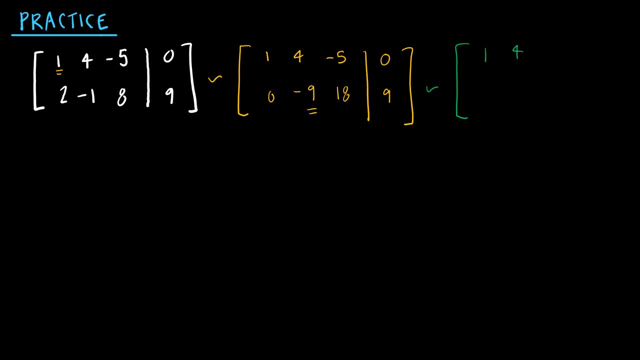 That's going to sorry, not everything. I'm going to take row 2 times negative 1. 9th row 1.. I would not do that too. This gives me 0, positive 1, negative 2, negative 1.. 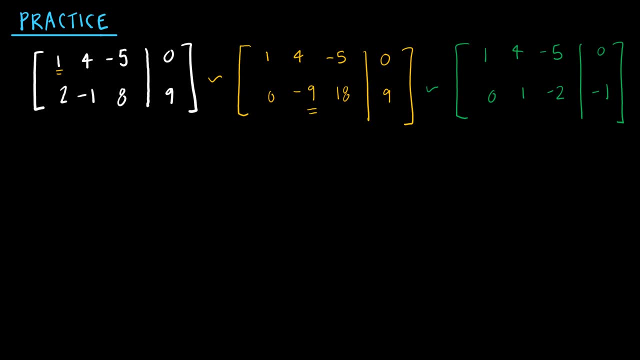 From here I'm trying to then turn- um- let me find a different color guy- into a 0, because I want anything above or below a pivot to be 0. so I'm going to take negative 4 times Row 2 and add it to Row 1. so this guy I'm going to. 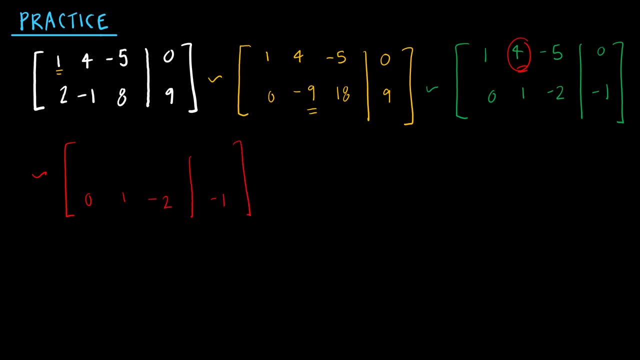 just leave alone and negative 4 times 0 plus 1 is 1. negative 4 times 1 plus 4 is 0. negative 4 times negative. 2 is 8 plus negative. 5 is 3. negative 4 times negative. 1 is positive 4 plus 0. so that's where I stand now. from here, keep. 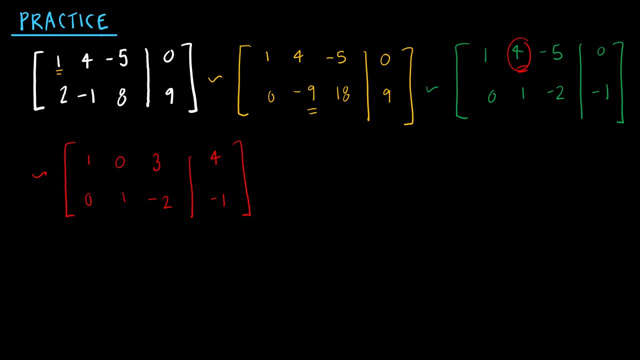 in mind what this is telling me. I have X 1 plus 3, X 3 is equal to 4 and X 2 minus 2, X 3 is equal to negative 1, and if I want to write this in the proper format, I'm going to just: 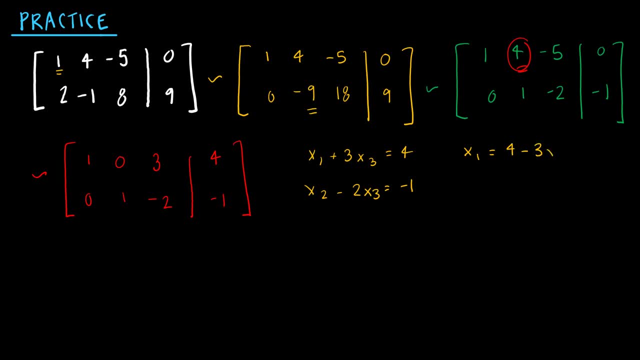 rearrange this so that X: 1 is 4 minus 3 X 3 X 2 is negative, 1 plus 2 X 3. so my solution: again written X 1, X 2, X 3, because obviously there are 3 X's would.